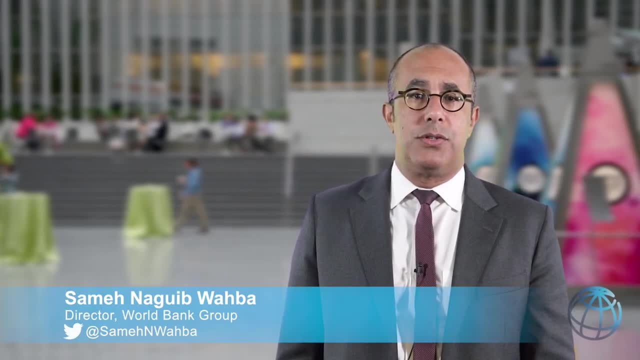 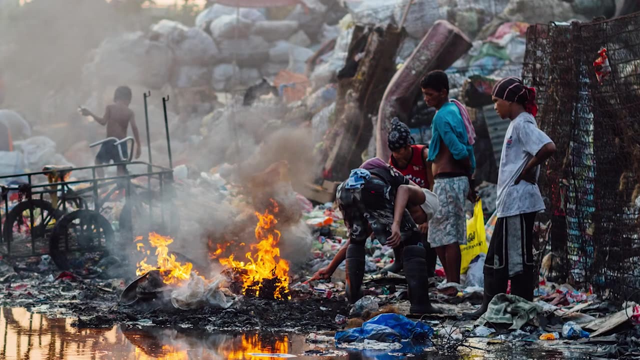 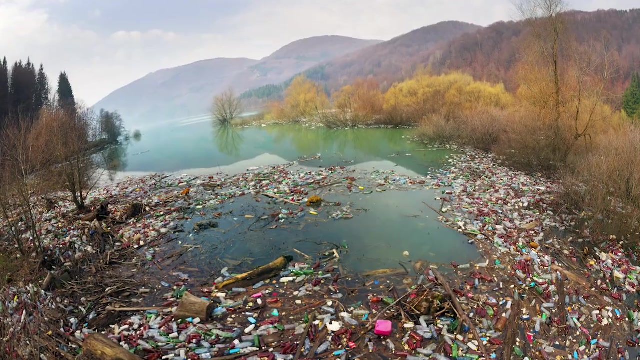 Poorly managed waste is contaminating the world's oceans, clogging drains and causing flooding, transmitting diseases, increasing respiratory problems from burning, harming animals that consume waste unknowingly, and affecting economic development, such as through tourism. Without urgent action, these issues will only get worse. 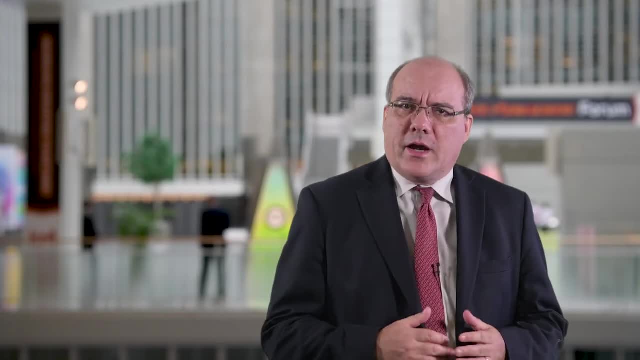 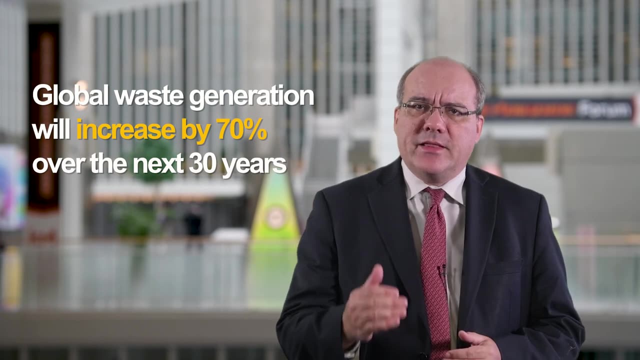 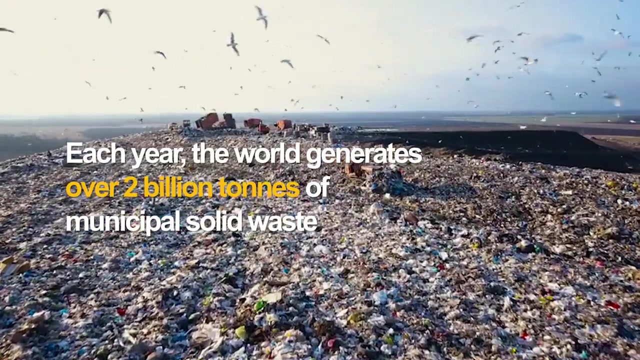 Here's what everyone should know. First, rapid urbanization, population growth and economic development will push global waste generation to increase by 70% over the next 30 years. Each year, the world generates more than 2 billion metric tons of municipal solid waste. Without urgent action, the global waste generation will increase by 70% over the next 30 years. Each year, the world generates more than 2 billion metric tons of municipal solid waste. Without urgent action, the global waste generation will increase by 70% over the next 30 years. 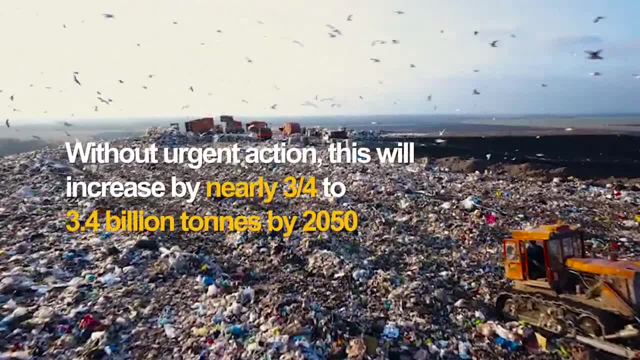 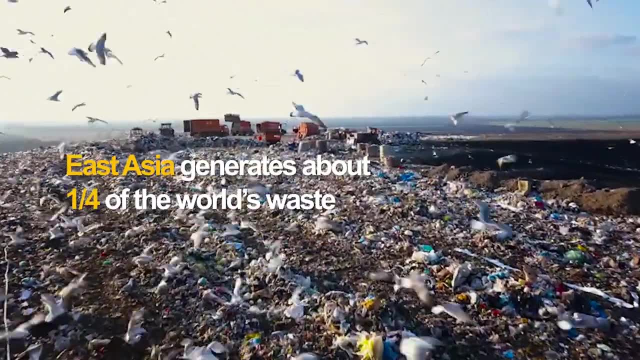 Each year, the global waste generation will increase by 70% over the next 30 years. With rapid urbanization, this will increase by nearly three quarters to 3.4 billion tons over the next 30 years. East Asia currently generates about one quarter of the world's waste, while waste generation 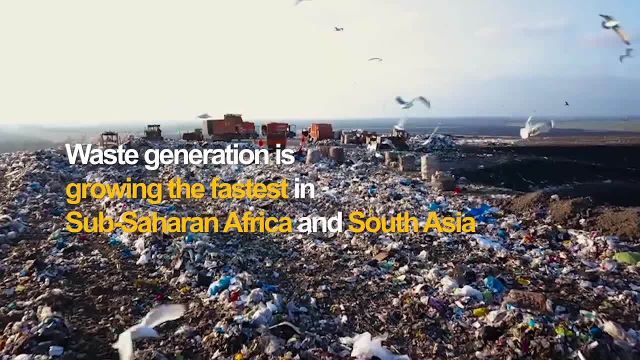 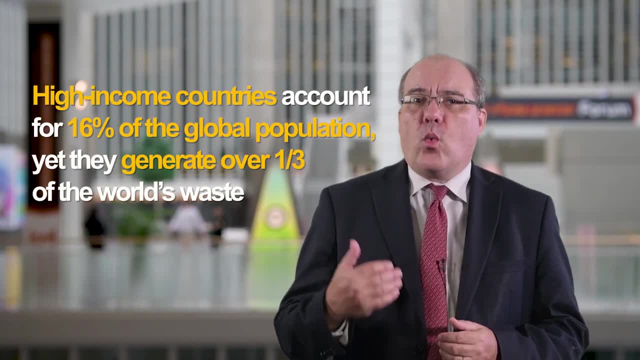 growing the fastest is in Sub-Saharan Africa and South Asia. While high-income countries account only for 16% of the global population, they generate over one-third of the world's waste. Second, in low-income countries, over 90% of the world's waste is generated by the. government – and they're 50% of the world's waste. Third, in low-income countries. 80% of the world's waste is generated by the government – and 90% of the world's waste is generated by the government itself. 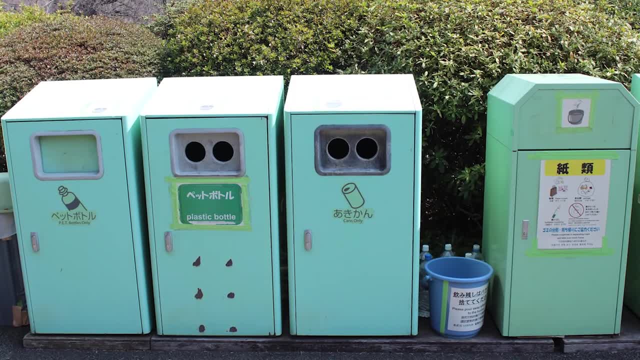 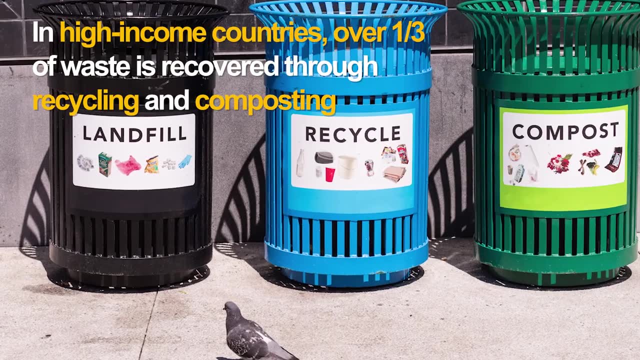 In some countries. more than one-third of the world's waste is called waste. It's either openly dumped or burnt. It's neither openly dumped nor burnt. Upper-middle and high income countries provide nearly universal waste collection. In high-income countries, more than one-third of waste is recovered through recycling and 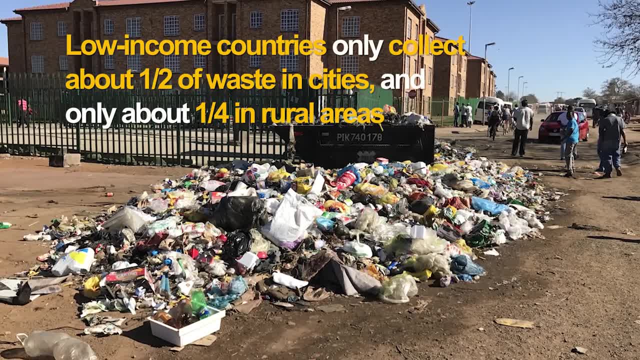 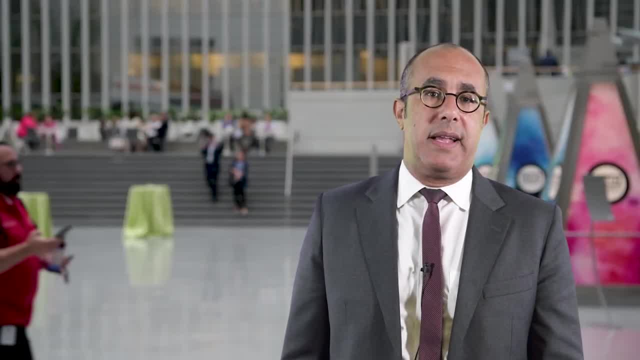 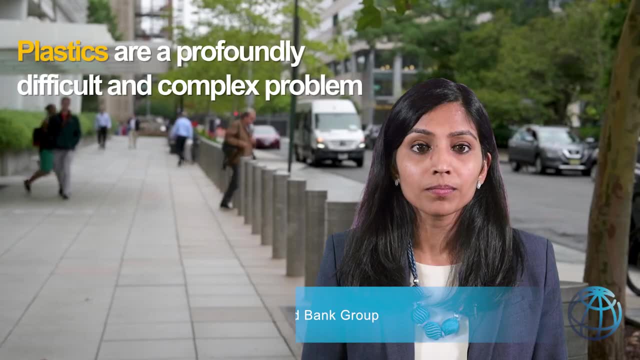 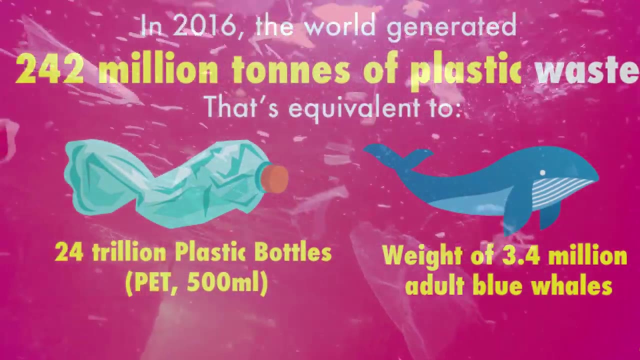 composting. Low-income countries only collect about half of the waste in cities and only about one-quarter in rural areas. There is much to be done in collecting waste in low-income countries. Third plastics are a profoundly difficult and complex problem. In 2016,, the world generated a whopping 242 million metric tons of plastic waste. 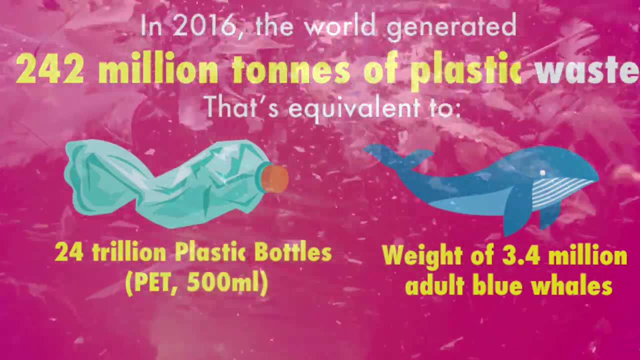 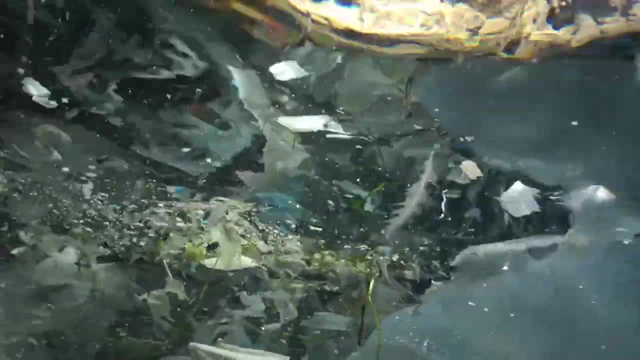 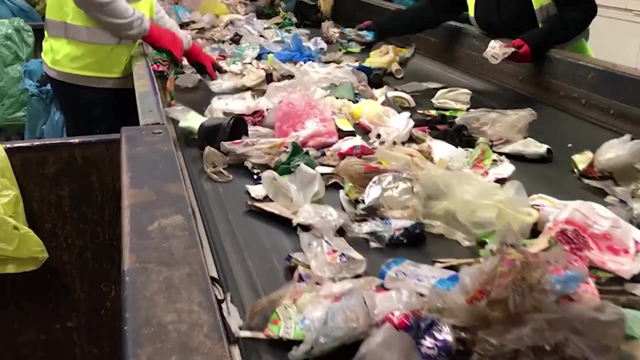 We could make about 24 trillion plastic bottles out of it, and their water volume could fill up to 4.8 million Olympic-sized swimming pools. Even when plastic waste is collected, many countries don't have the capacity to process the waste, leading to dumping or mismanagement of it. 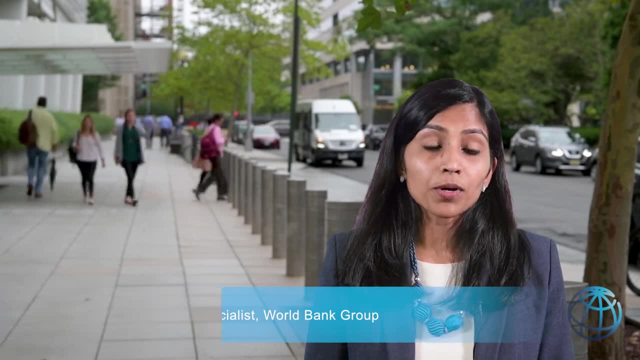 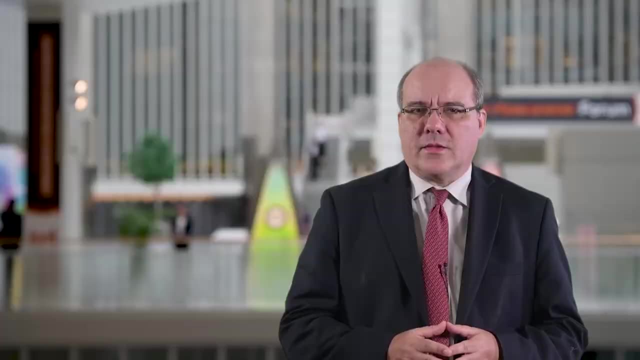 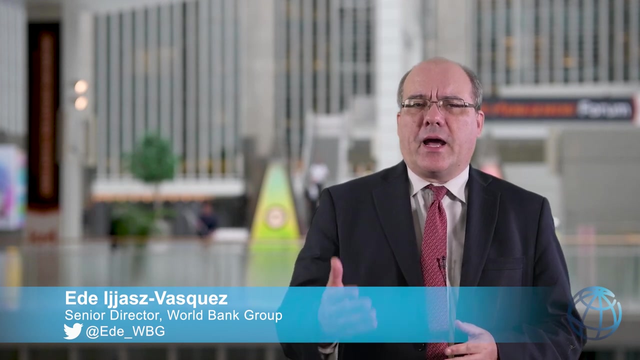 Plastics in rivers, waterways and oceans are a particularly growing, urgent problem. Ninety percent of marine debris is plastic. Waste is growing, but so too is the global momentum to find solutions to stem the tide and make waste management more sustainable. 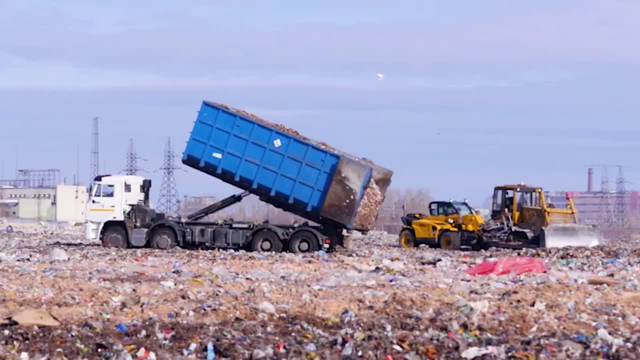 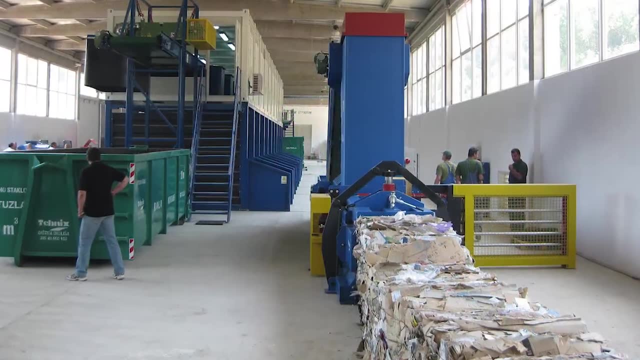 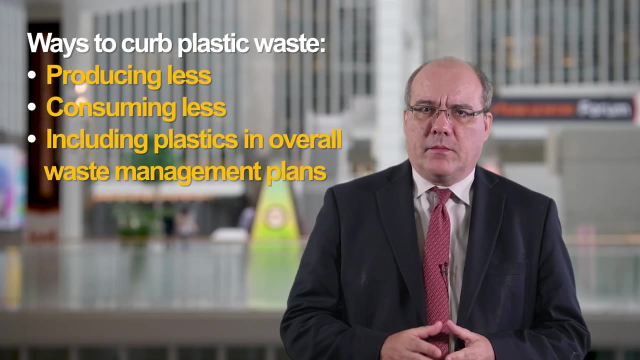 Many solutions already exist. The World Bank is increasingly working with developing countries worldwide to invest in sustainable waste management to address challenges related to infrastructure, governance, financing and capacity. For example, there are different ways to curb plastic waste by producing less consuming. 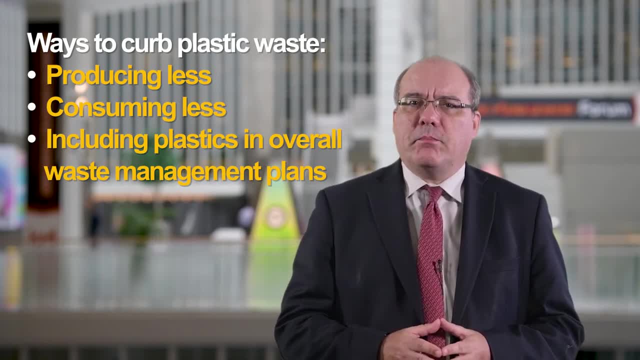 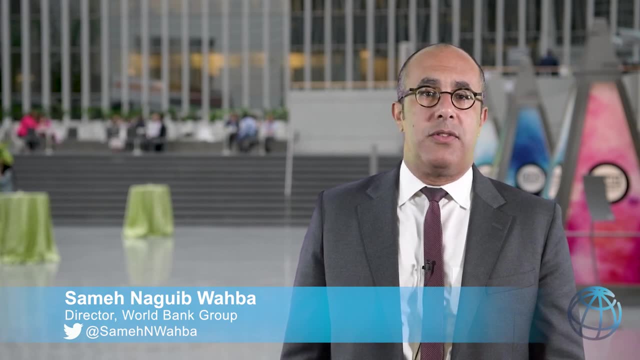 less and including plastic in overall waste management plans. Solid waste data and planning are also part of the solution. It is important to understand that plastic waste is a very important part of the solution. We need to understand how much and what types of waste are generated and where. 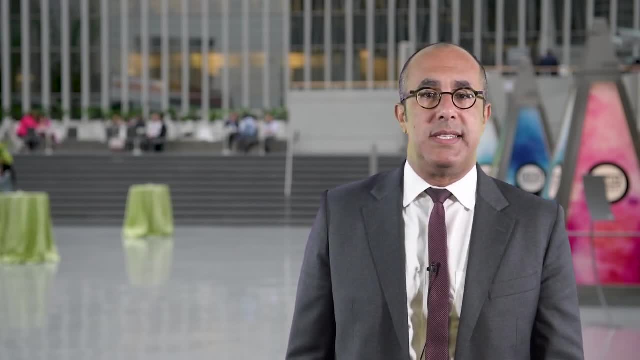 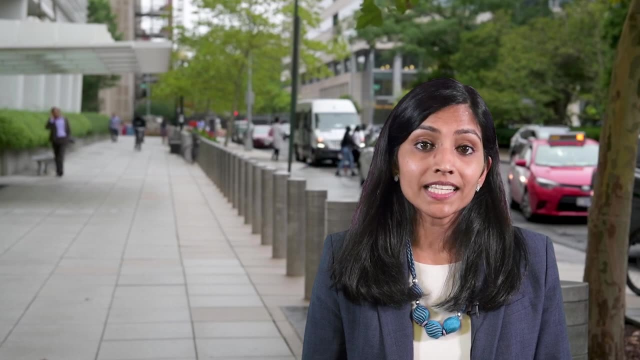 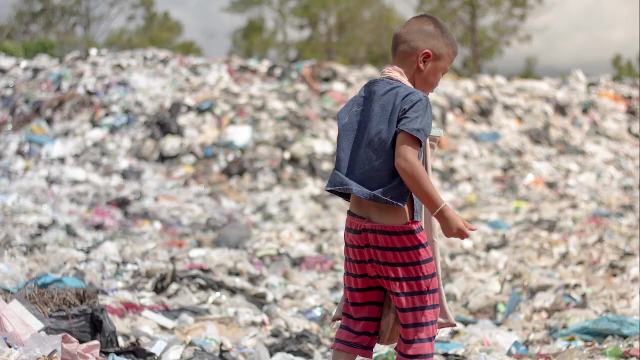 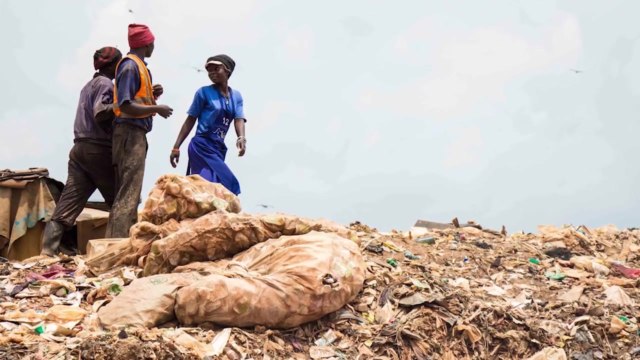 This can help governments create more effective waste management policies and plans for the local context. Waste management can be costly. It may be the single highest budget item for many local governments. However, it makes economic sense to manage properly. Uncollected waste and poorly disposed waste have significant health and environmental 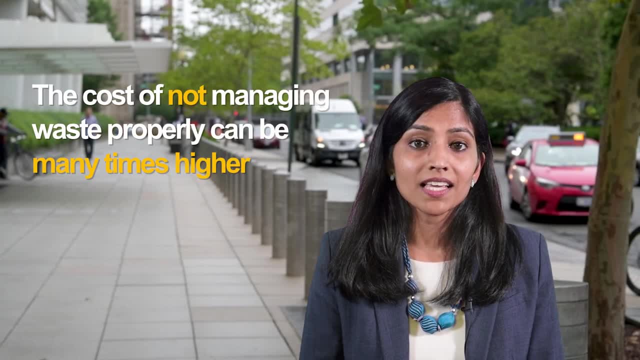 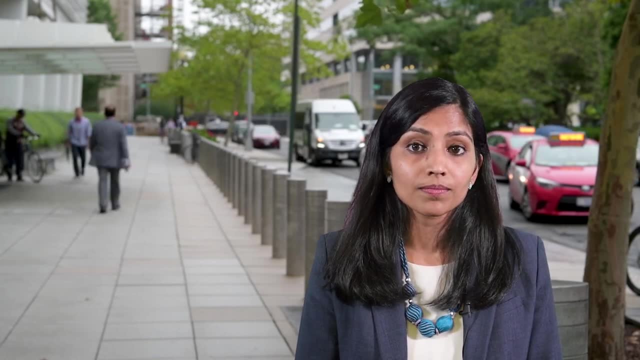 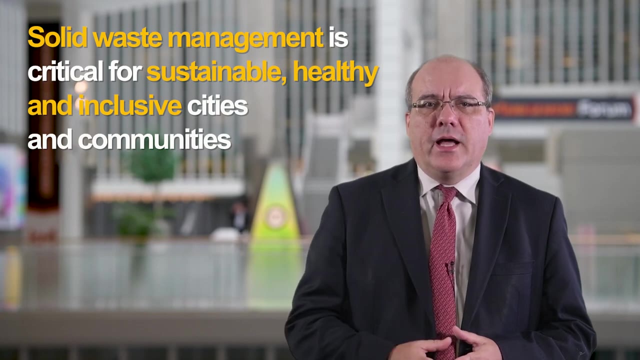 impacts. The cost of addressing these impacts is many times higher than the cost of developing and operating simple, adequate waste management systems. In an era of rapid urbanization and population growth, solid waste management is a critical piece for sustainable, healthy and inclusive cities and communities. 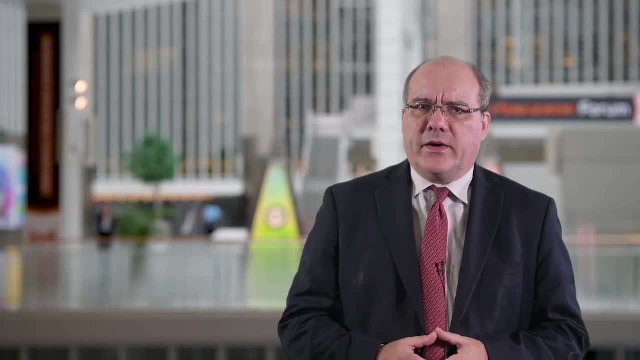 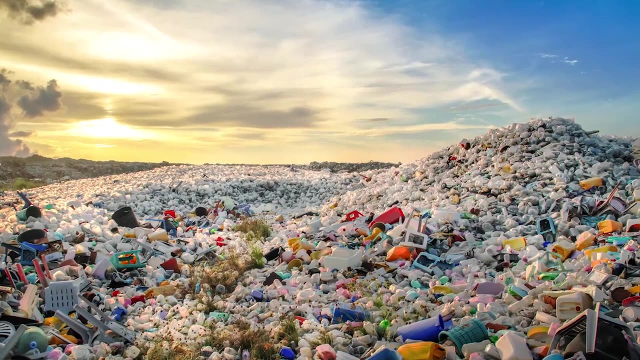 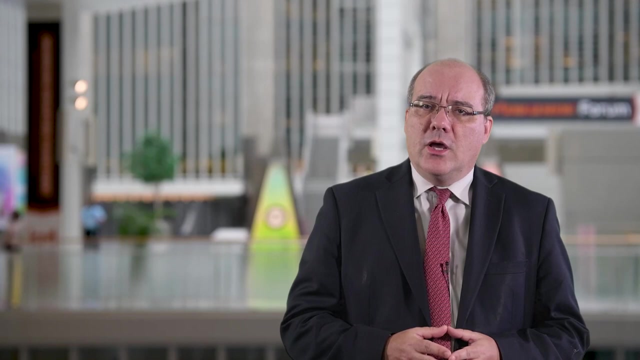 However, it is often put on the back burner when it comes to urban development. If no action is taken, we will push ourselves and our children to live in a world with more waste and overwhelming pollution. Lives, livelihoods and the environment will pay an even higher price than they are already. 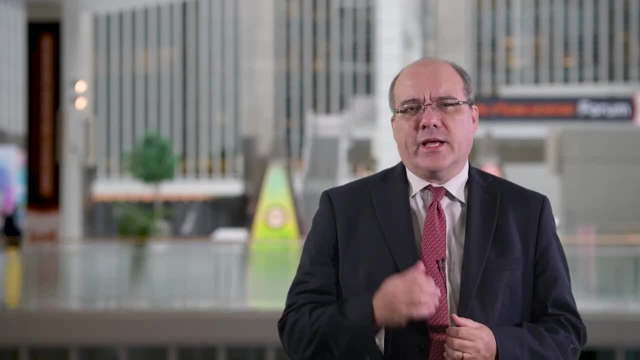 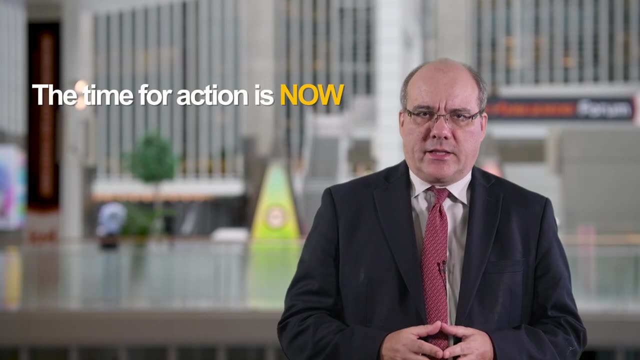 We already know what needs to be done to reverse that trend. We just need all levels of society to take urgent action. Sustainable waste management is everyone's business. The time for action is now.